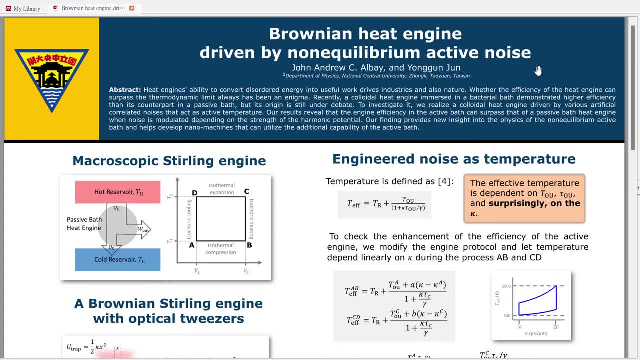 Brownian heat engine driven by non-equilibrium active noise. As we know, heat engine converts a percentage of the energy from hot reservoir into work, and this fraction is the engine's efficiency. One example of a heat engine is the Stirling engine and right now, a Brownian. 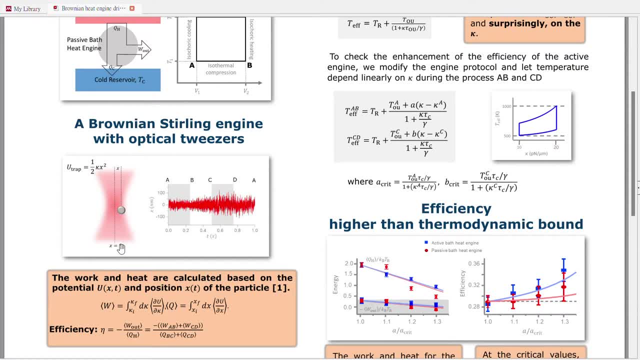 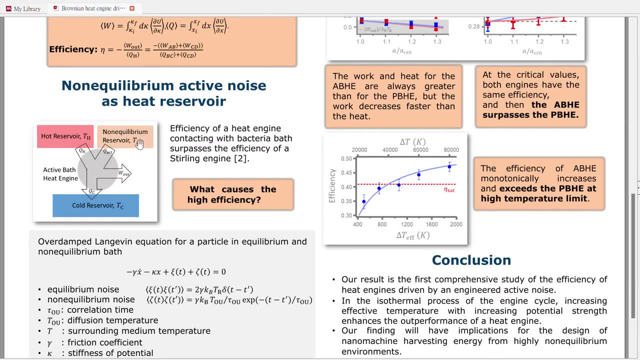 Stirling engine is easily realized with an optical tweezer and well explained by the stochastic thermodynamics. The focus now is on utilizing non-equilibrium active noise as heat reservoir, and one recent experiment shows that the efficiency of a heat engine contacting with a bacteria bath surpasses that of the Stirling engine. As a motivation, 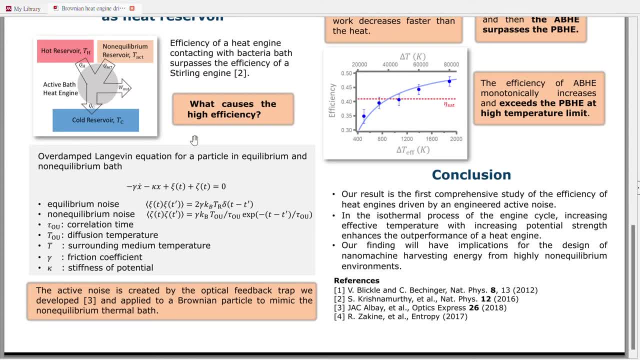 for our work. we want to understand what causes the high efficiency. In able to do this, we apply an active noise that is exponentially correlated to a Brownian particle To mimic the non-equilibrium active bath, and it is easily created by the optical feedback. 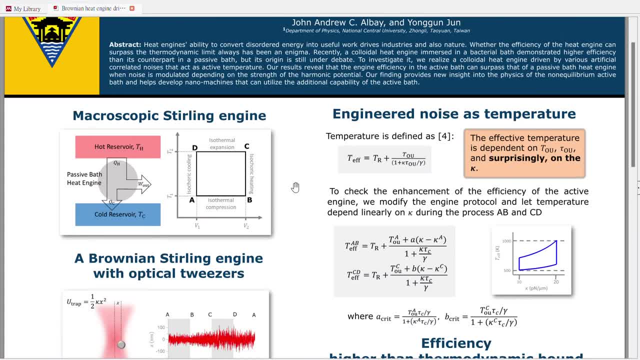 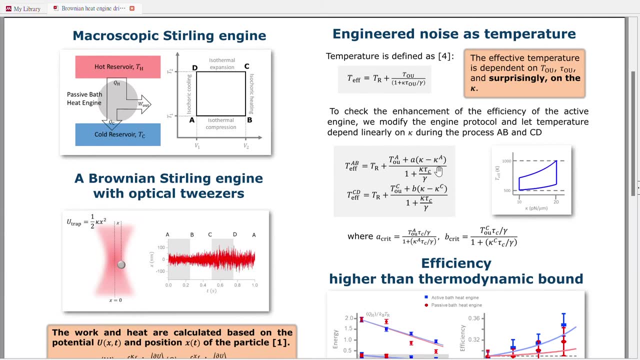 trap we develop. The effect of the noise is quantified as temperature and it is dependent on the amplitude and correlation of the noise and, surprisingly, on the stiffness of the potential. So to check the enhancement of such engine, we modify the protocol and let temperature 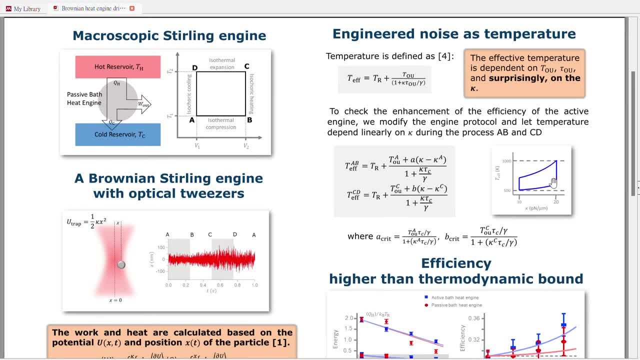 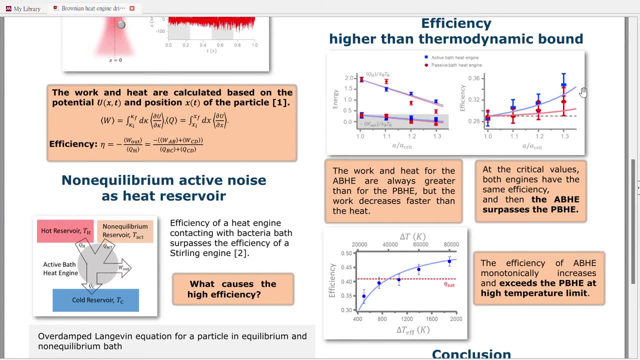 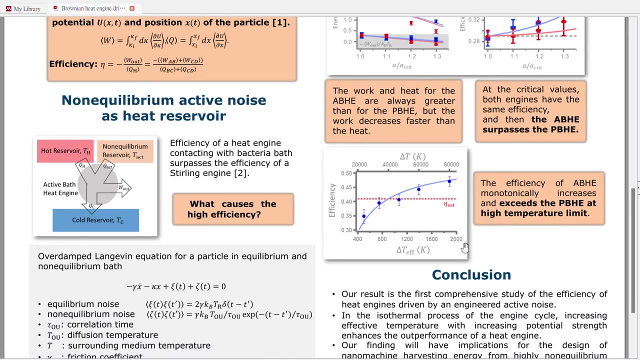 depend linearly on the stiffness during the isothermal process. So after checking the work and heat, we found that the efficiency of an active bath heat engine surpasses that of a passive bath heat engine. And also, even at high temperature limit, we found that the active bath heat engine's efficiency exceeds that of the saturated 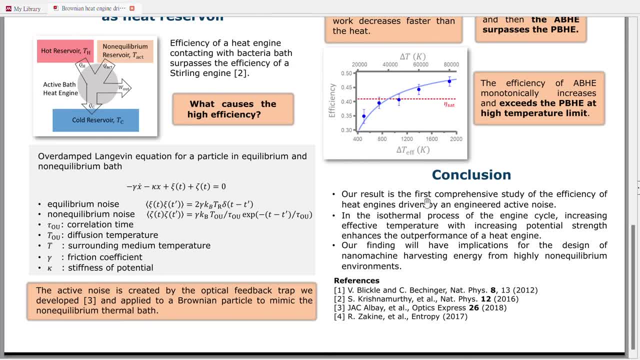 efficiency of the passive bath heat engine. So, as a conclusion, our result is the first comprehensive study of the efficiency of heat engine driven by active bath heat engine. In addition to an engineered active noise, our finding will have implications for the designs of nanomachines harvesting energy from highly non-equilibrium environments.